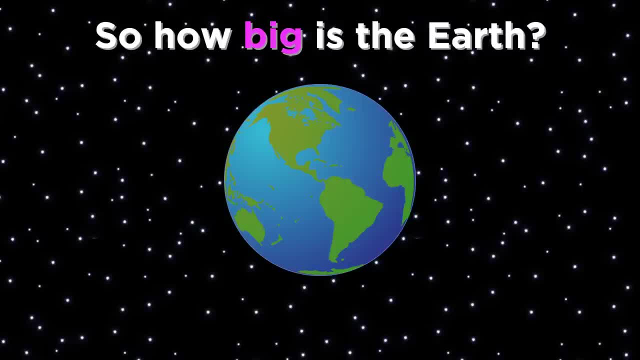 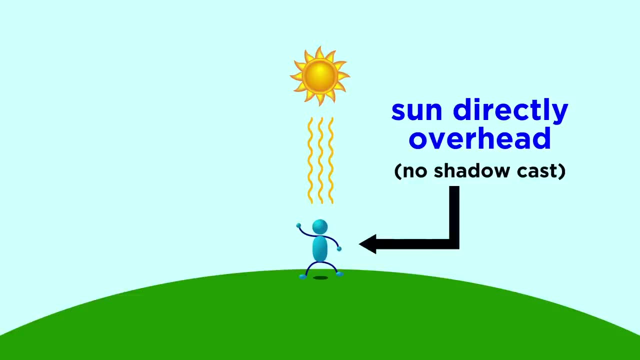 attempt to measure the dimensions of the sphere. Eratosthenes was the first to do this, and with impressive accuracy. He reasoned that when the sun is directly overhead one object, it must cast a shadow on some other object sufficiently far away. 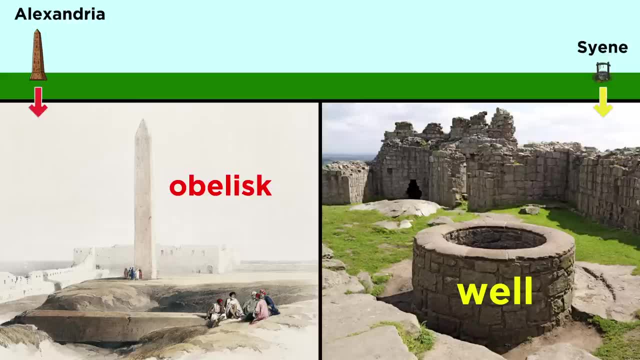 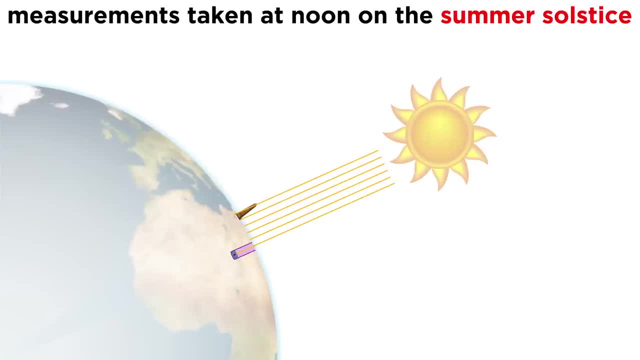 He used a well in one part of Egypt and an obelisk in another part of Egypt to measure the dimensions of the sphere. At noon on the summer solstice, the sun shone directly down the well, illuminating the very bottom. 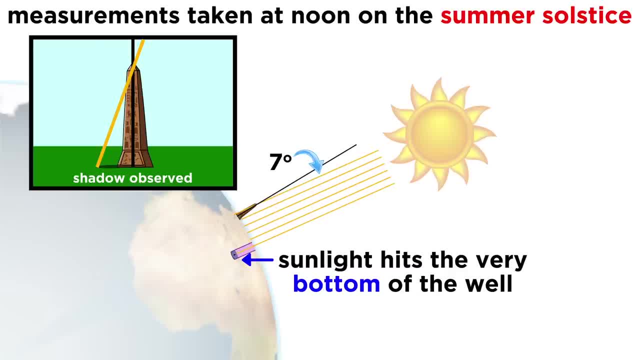 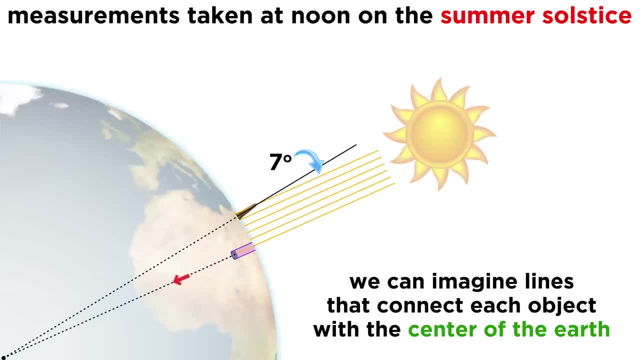 Simultaneously, the sun cast a shadow on the obelisk in Alexandria, revealing that the sun was seven degrees off the vertical. Now let's draw a line from the bottom of the well to the center of the earth and another one back up to the base of the obelisk. 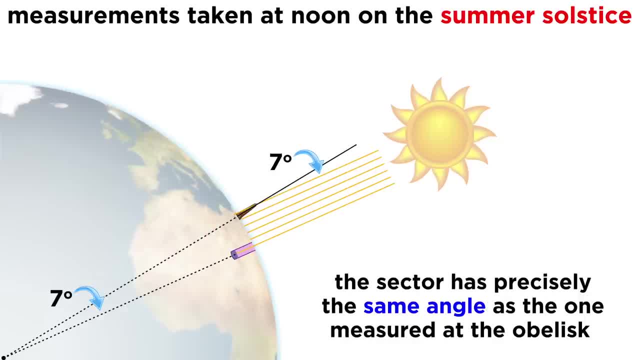 By simple geometry, the sun is not directly overhead. If we draw a line from the bottom of the tree, we can see that the angle of this sector is seven degrees, which means that this distance represents a little less than a fiftieth of. 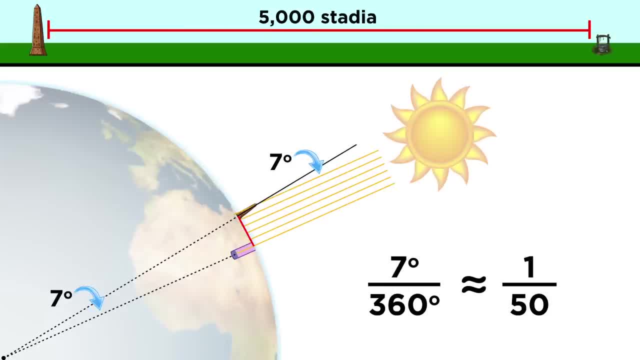 the way around the world. The distance between these locations was known to be five thousand stadia, so we can use a simple ratio to deduce that the circumference is around two hundred fifty thousand stadia, which is around twenty-five thousand miles, Given that in ancient times the over-the-top receiver around the top bottom could be particularly 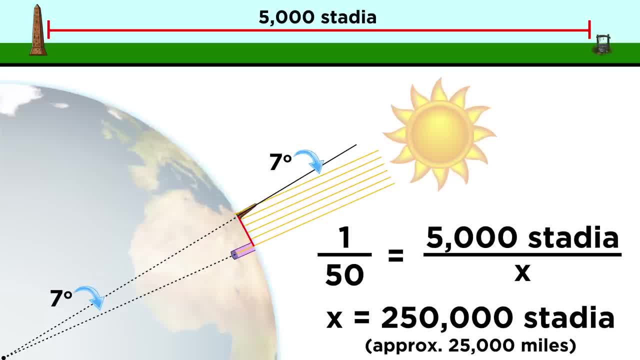 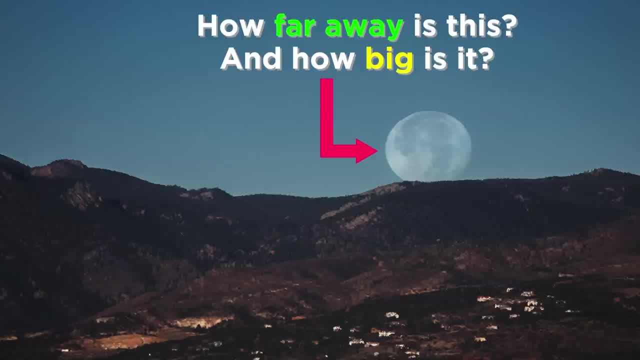 the only tool available was the naked eye. these are all demonstrations that you can reproduce yourself, in case you're curious to try. Now that we are all set with the earth, what about the distances to other objects in the sky, And how big are those? 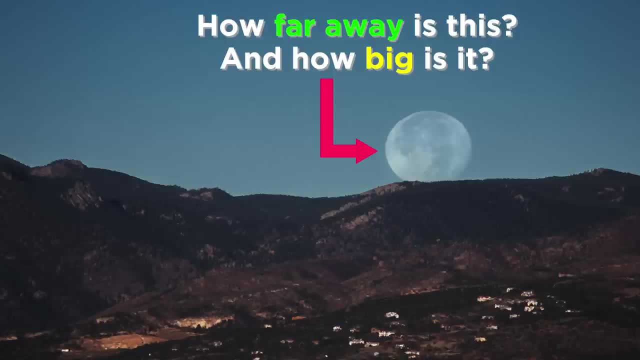 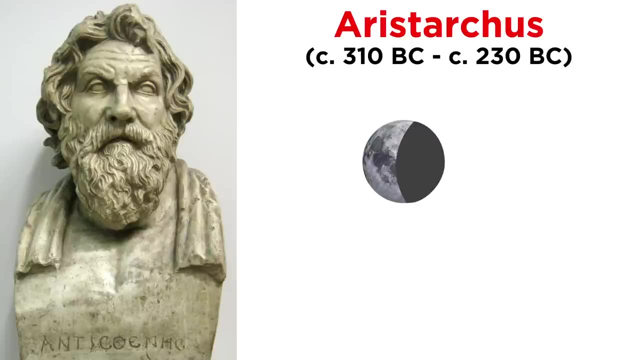 Incredibly, we were able to deduce some of these quantities as well. Take the moon, for example. Around the time of Eratosthenes, another Greek named Aristarchus did some similar work. He looked at the shadow of the earth on the moon during a lunar eclipse and by comparing, 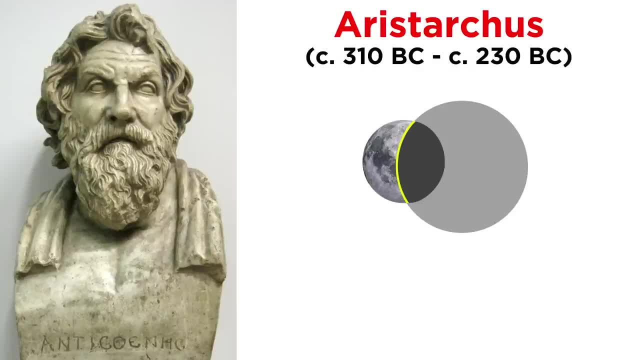 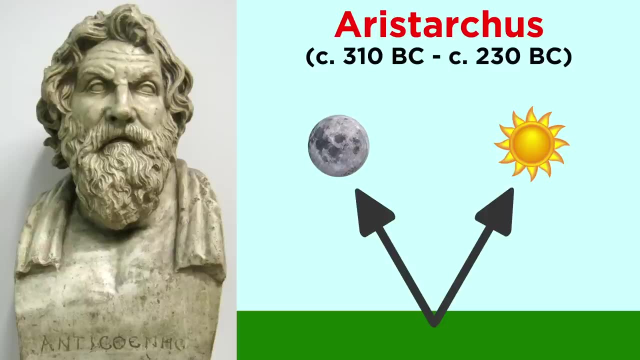 the curvature of the shadow and the moon itself, he deduced that the moon must have a diameter around one third that of earth. He also made estimates regarding the relative distances to the moon and sun, and although those were not as correct as his other work, he was the first.